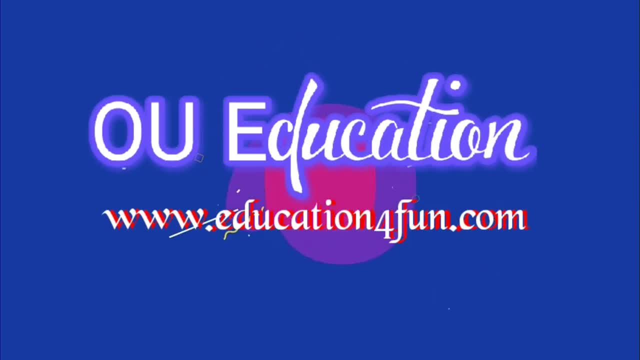 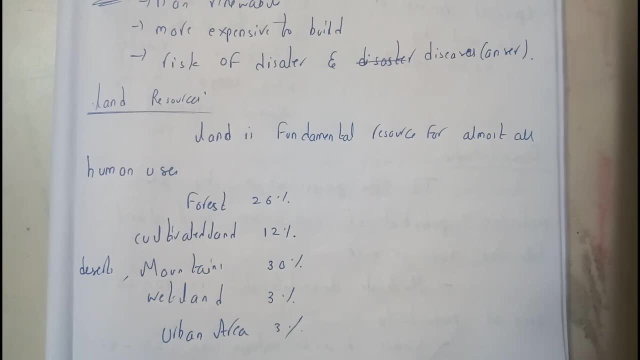 In this tutorial let's see about land resources and we'll be discussing about soil pollution and desertification. These are the last three topics in this chapter, So we'll try to complete in this tutorial. So, basically, what is land resource? Land is a fundamental resource for. 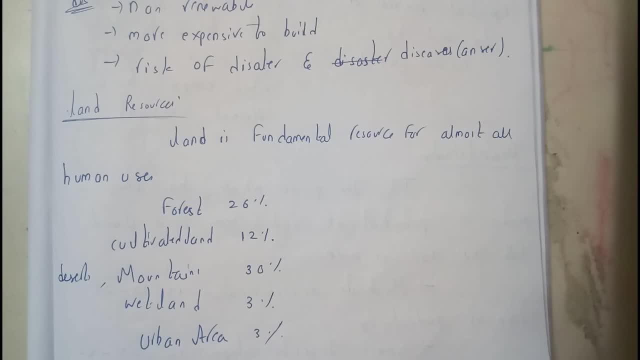 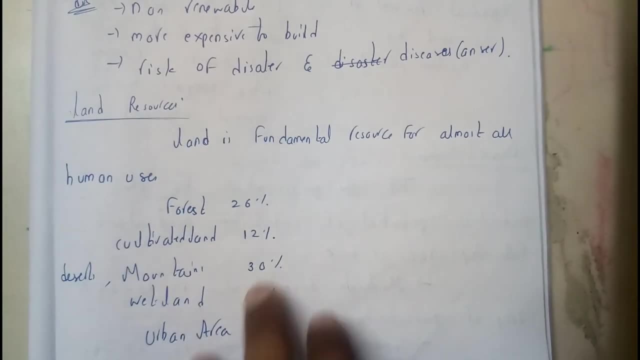 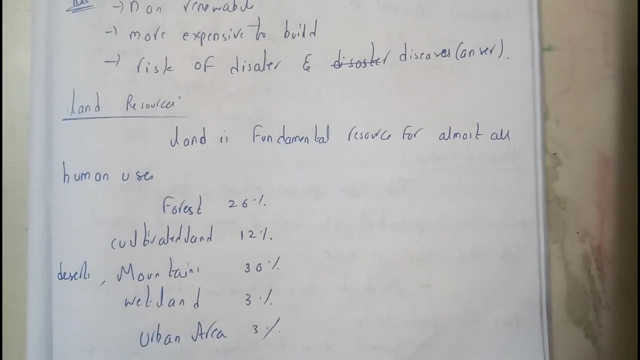 almost all human beings. We live on the surface of the earth, which is land. So forest is covered by 26 percentage and cultivated land will be 12.. Deserts and mountains is 30 percent and wetland is 3 percent and urban area is 3 percent. So I hope everyone got a small idea on what is land. 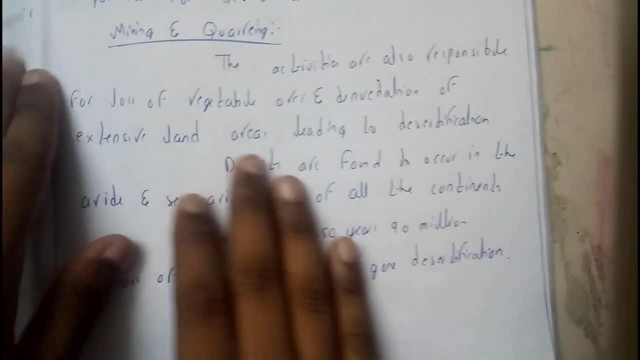 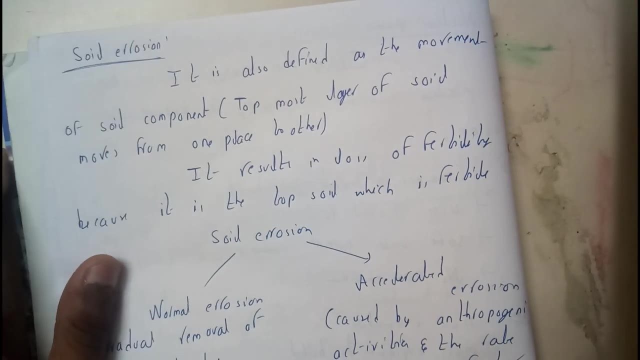 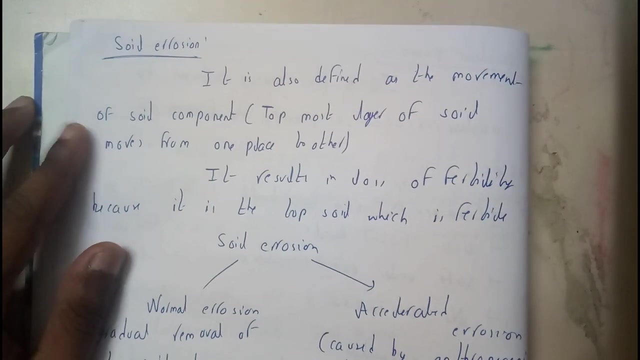 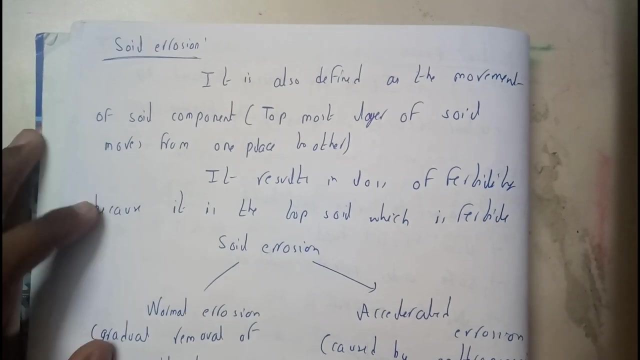 resource. So this is all up to land resource and whenever we are going through land means we are. that means soil erosion, we gonna, we should get remember. So soil erosion. It is also defined as the movement of soil components, which is not but the top most layer of soil moves from one place to another- is soil pollution. 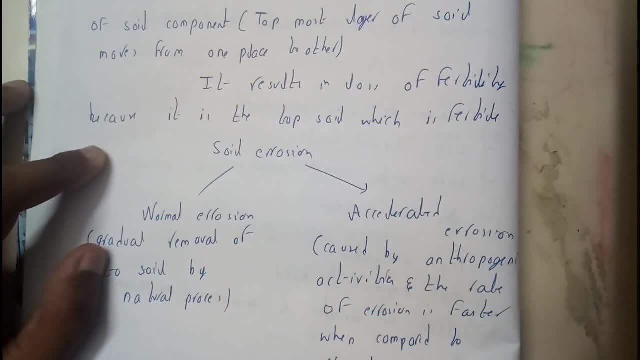 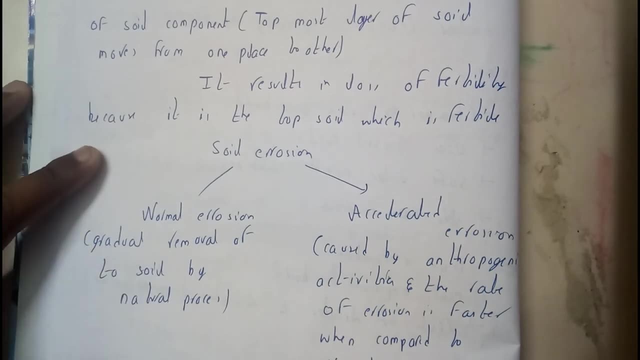 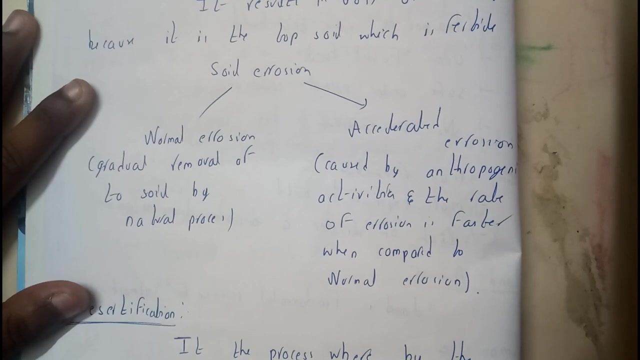 So it refers in the. it refers in the loss of fertility because it is the top, so top soil which is fertile. I think around 2.5 centimeters is the most fertile land, Most fertile land, Most fertile surface of the land. So soil erosion is again further divided into two. 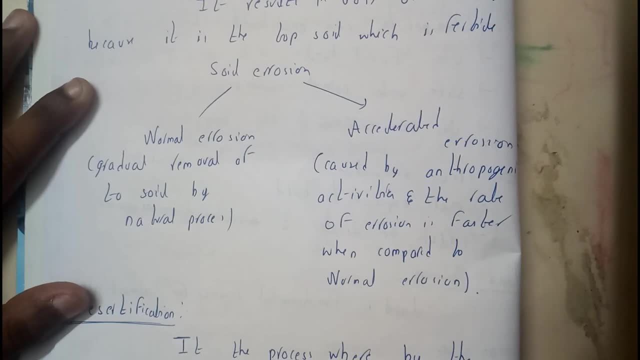 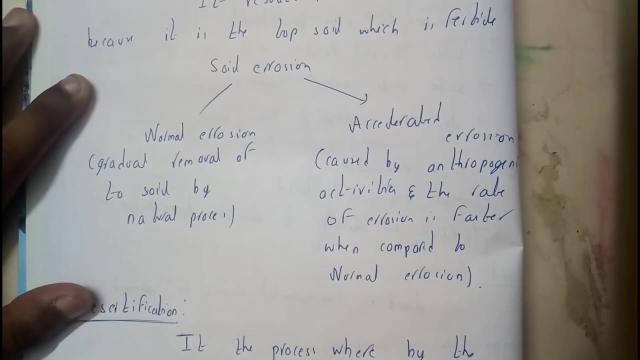 types. One is normal, another one is accelerated. Normal is a natural process which is really slowly occurring process, And accelerated is nothing but it is due to man or human. This type of accelerated is very, very faster when compared to normal. So I hope everyone. 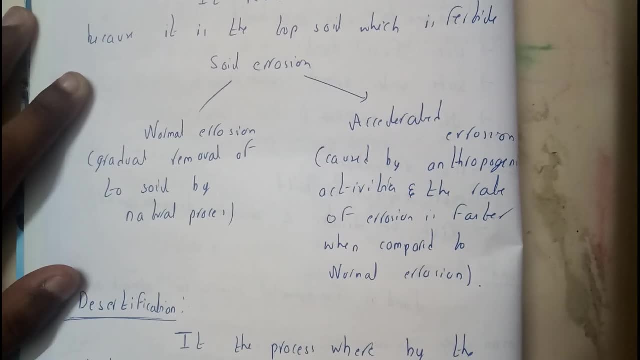 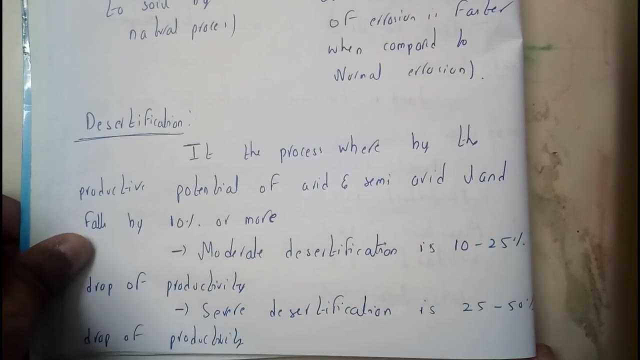 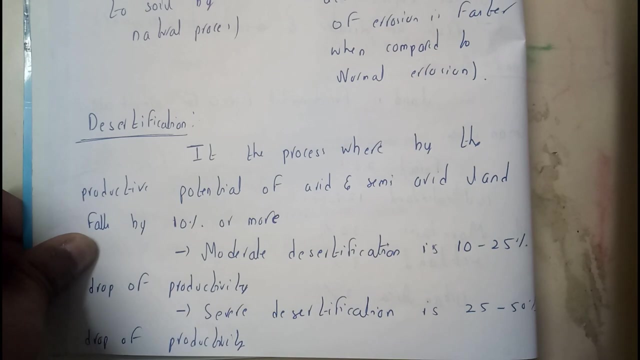 is now clear with what is land resource And soil erosion. And now let's see what is decertification. Decertification is nothing, but it is the process whereby the productivity potential of arid and semi-arid area lands falls by 10% or more. 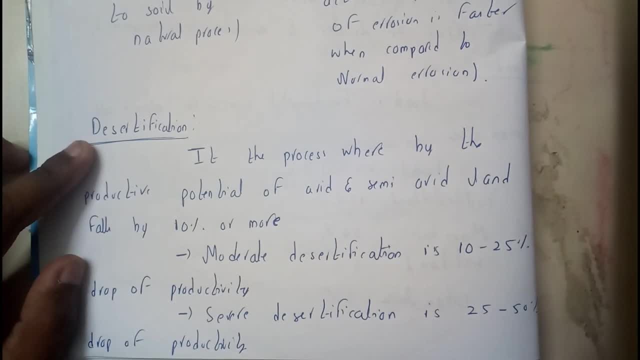 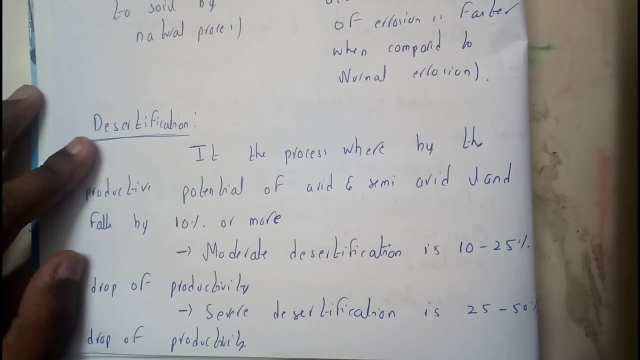 Okay, I hope you got a small idea on decertification. If the decertification, if the decertification is more in between 10 to 25%, Okay, Okay, It is called moderate decertification and it is 25 to 50, it is severe decertification.